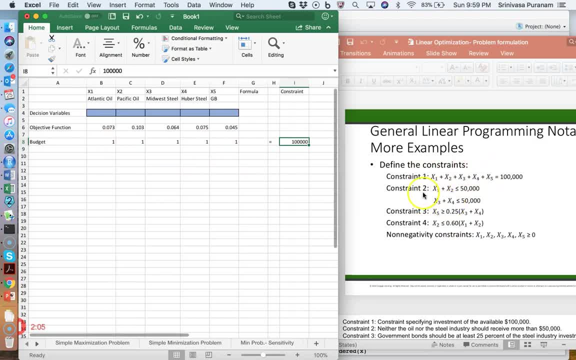 three, when there are no coefficients. the coefficients are essentially one. one times the number is the same number. okay, we cannot have more than 50 000 invested either in oil or in steel. uh, no more than 50 k in oil. so you have x1 plus x2 is less than equal to 50 000. 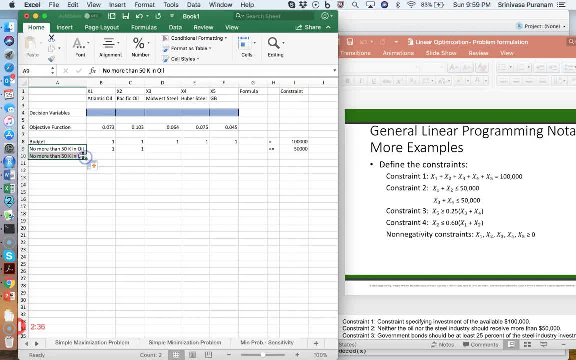 then you have no more than 50k in steel. that's x3 plus x4, less than or equal to fifty thousand. now, uh, constraint three here. this is a greater than constraint, because we already wrote two less than or equal to constraints. i'm going to write constraint four first. 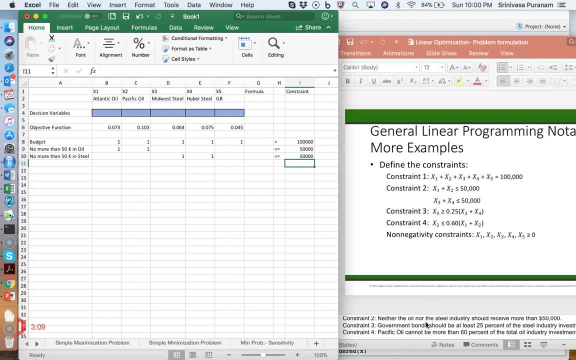 um, this constraint, uh says that pacific oil cannot be more than 60 percent of the total oil industry investment. so i'm going to write that constraint first, pacific oil constraint, and that says so. now you have a couple of options. so the options are here. it says x2 is less than or equal to 0.6 times. 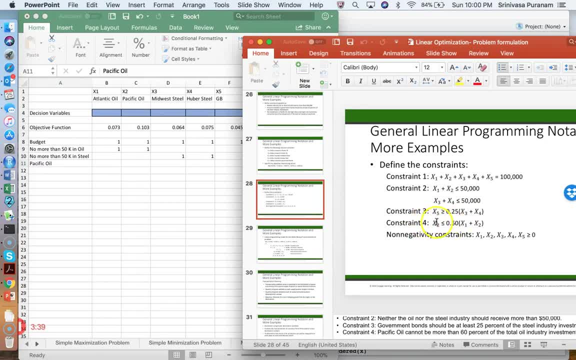 x1 plus x2, so you have x2 on the left hand side, you have x2 on the right hand side. now, the traditional way to do this is you collect all variables on the left hand side and you only put numbers on the right hand side. so what this will transform to: 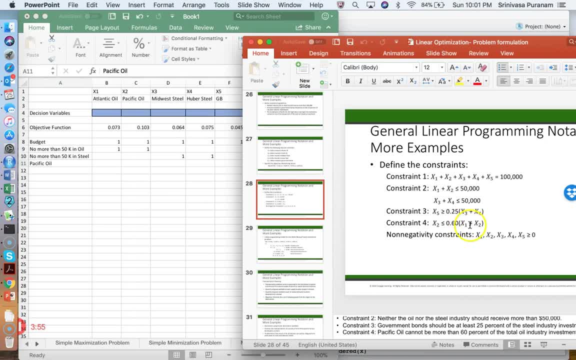 essentially is you have 0.6 times x1 here plus 0.6 times x2 and you transfer all of this to the other side of the constraint and they become negative. so you get negative. 0.6 times x1 negative. 0.6 times x2 plus x2 is less than or equal to zero, so negative. 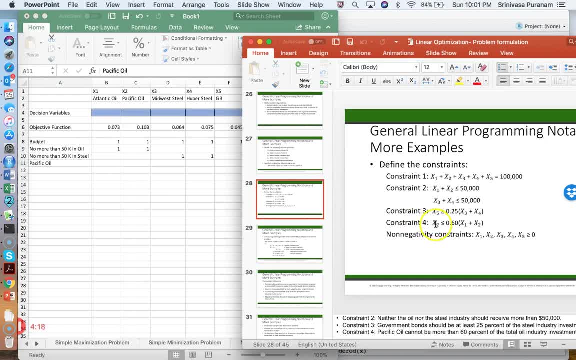 0.6 times x, x2 plus x2, that becomes positive point for x2. so you can simplify this constraint further. but you don't have to. you can just leave it the way it is, and i'm going to type it just the way it's. 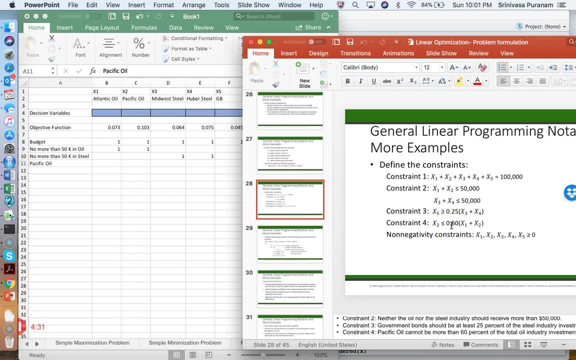 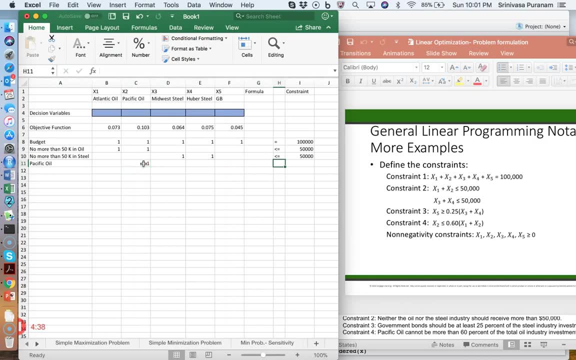 written here. so it says x2 is less than 0.6 times x1 plus x2. in parenthesis, this says x2 is less than or equal to. now, because you have to write a formula here, i'm going going to begin that with an equal to, so 0.6 times X 1 plus X 2, we say X 1 plus X. 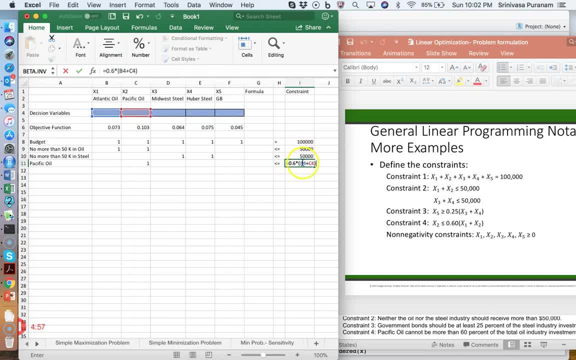 2, and this is where you have to be careful. it's very common I've seen students make the mistake where you choose these two cells. here you cannot do that: X 1 and X 2. here they are the variables, so you have to choose X 1 and. 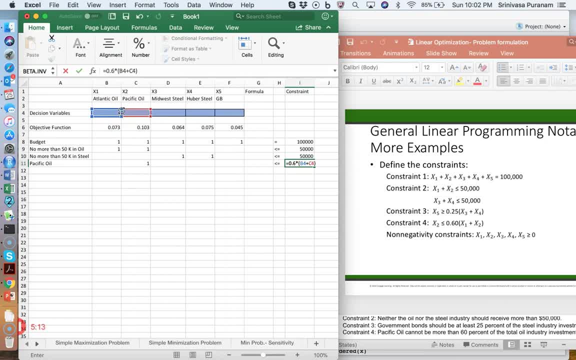 X 2 right from here. right, keep that in mind. okay, that's a specific oil constraint. and finally, of the government bond constraint. the government bond constraint is that common bonds should be at least 25% of the steel industry investment. so that's the constraint, so it's a greater than constraint, that's. 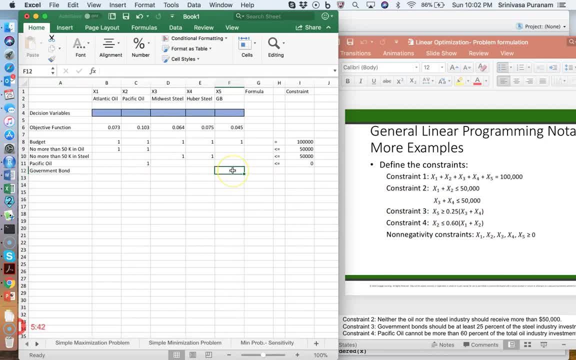 why I wrote it later. so it says X 5 is greater than or equal to 0.25 times. again it is X 3 plus X 4, so it is X 3 plus. forgot to put the equal sign. doesn't know, it's a formula: X 3 plus X 4. 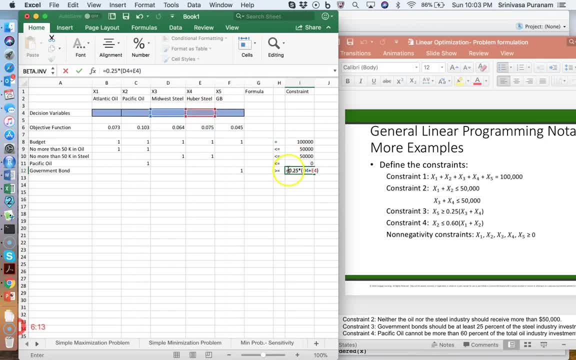 so don't forget the equal to sign, like it just did. if you don't, excel doesn't know that you're writing a formula. now, all the data here has been put in, except for the non-negativity constraints which obviously, as you know, we're going to put. 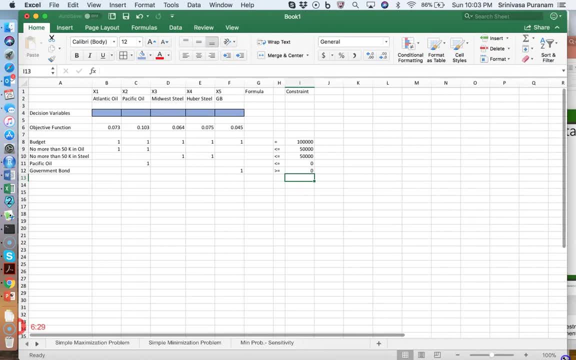 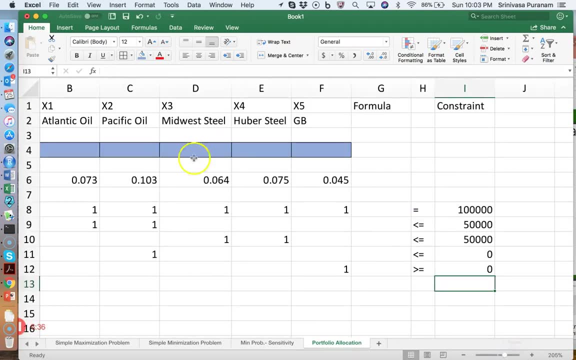 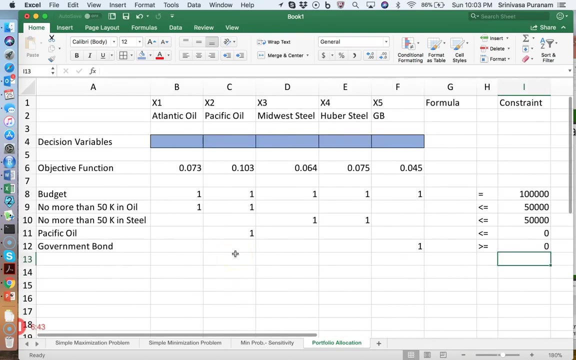 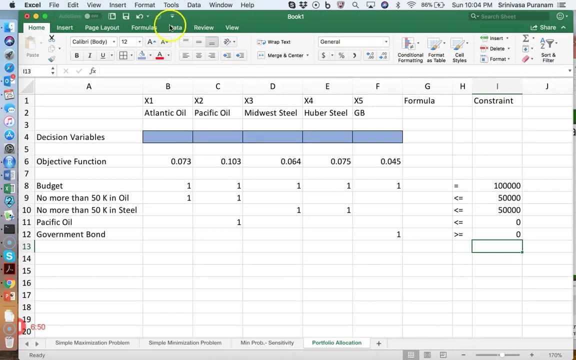 are we going to make? make it part of the solver tallow box. there you go. so all the formulas are here. everything is here. we can solve this problem. okay, you can bring up the solver dialog box. we go to data, bring up solver for the objective. ah, forget, we forgot. there are the 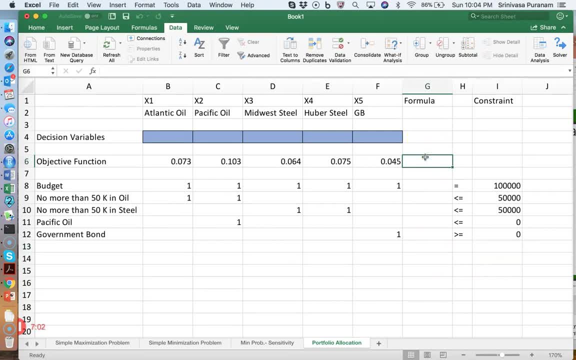 formulas, and this is where my way of writing formulas shines. so if I didn't write the formula, you have to do equal to and do this times, this plus this times, this plus this times. you want to do that for this. you do that for every one of. 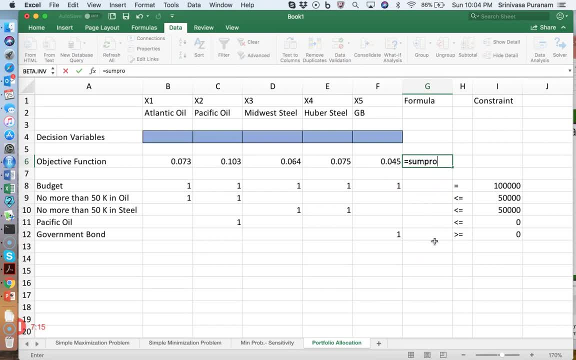 them. it makes a problem. instead, I can just write some product and I can say some product of this row, the coefficient row comma. all my decision variables and of course all my decision variables have to be absolute values, because in all my formulas, both for the objective function and all my constraints, I'm going to 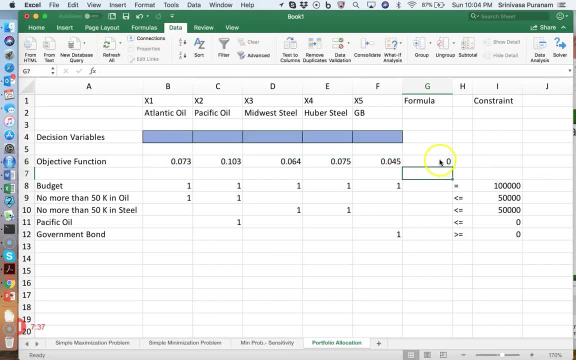 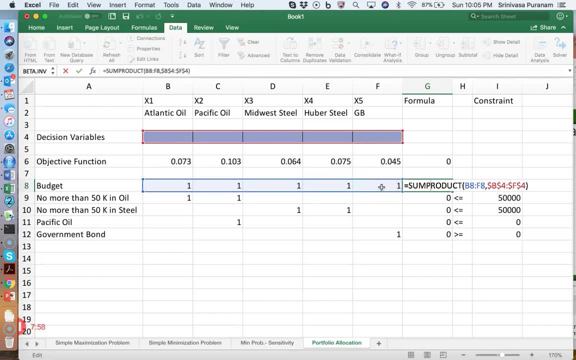 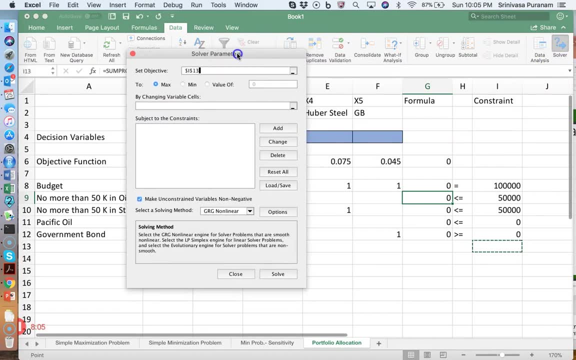 this number of this number and, finally, this number of this number and add them all up. okay, now that I have this, I'm going to put this in solver. I'm going to go through this quickly. in case you have a problem, you can either rewatch the 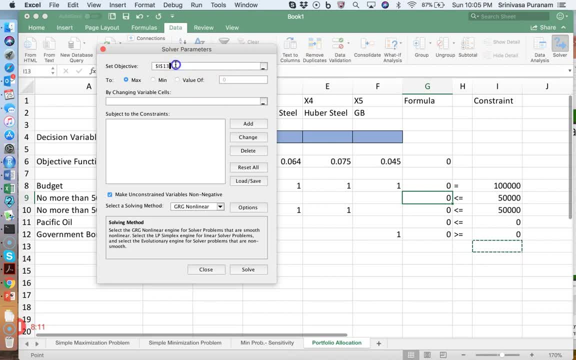 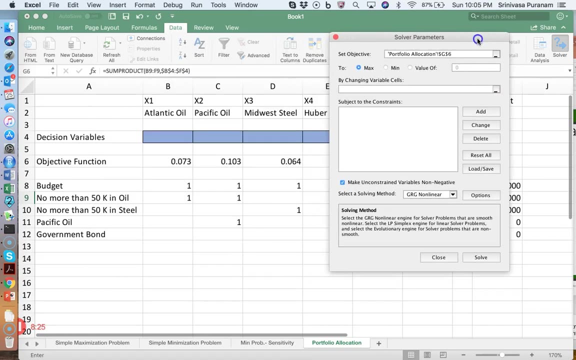 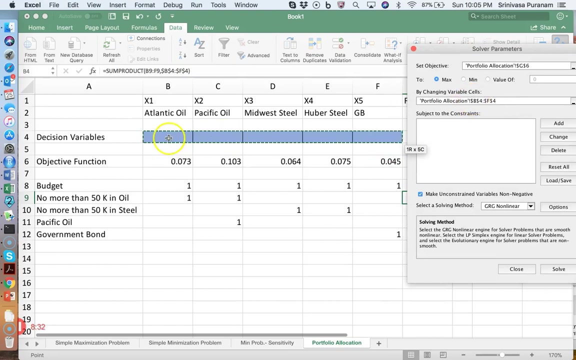 video or you can watch the minimization and the maximization videos, where I have spent more time. so the objective function is right there and there's a maximization problem. we are maximizing the returns, the changing variable cells. those are all my decision variables. so b4 to f4, these are all my decision. 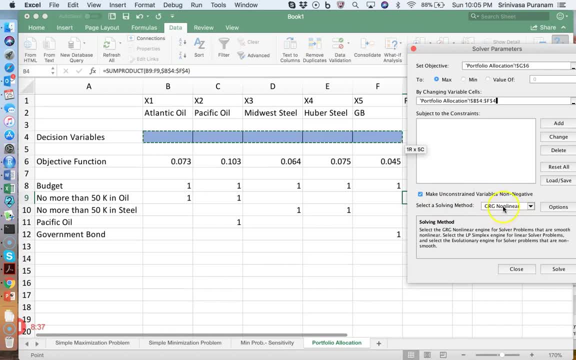 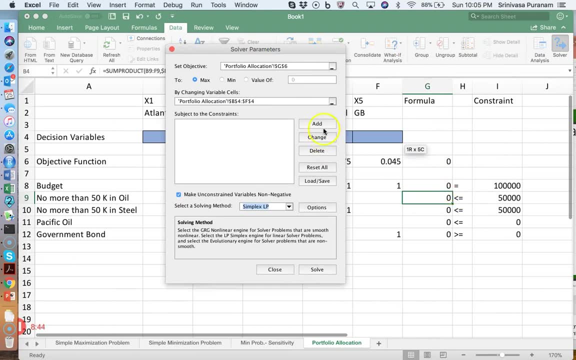 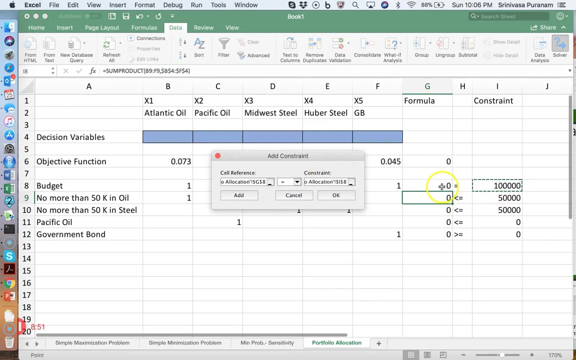 variables here. now let me write the constraints. oh, don't forget to change the solving method to simplex. okay, now we write the constraints. so first I'm going to write the equal to constraint. so I'm going to say that this left-hand side should be equal to this right-hand side, so g8 should be equal to i8. add. 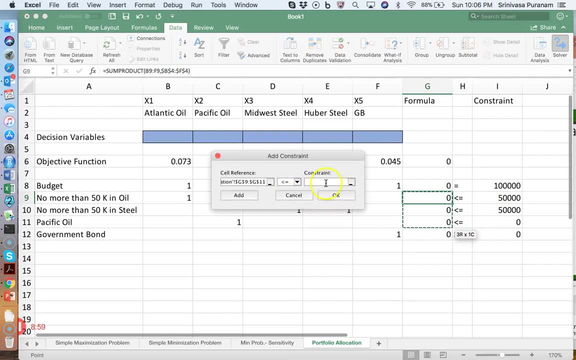 then all of these three left-hand sides have to be less than or equal to the corresponding values here. so again, there is a reason why I switched around these two constraints from the formulation, because I wanted to write all the less than or equal to constraints together. now. 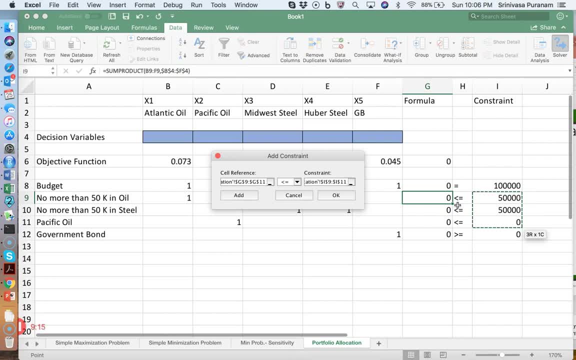 I'm writing in this way, it doesn't mean you have to do it this way. if you want to write each constraint separately, you will get the exact same solution. it is not different, so don't worry. worry about that. click Add. finally, write the greater than constraint. let's say, this number is greater than that number. click OK, so. 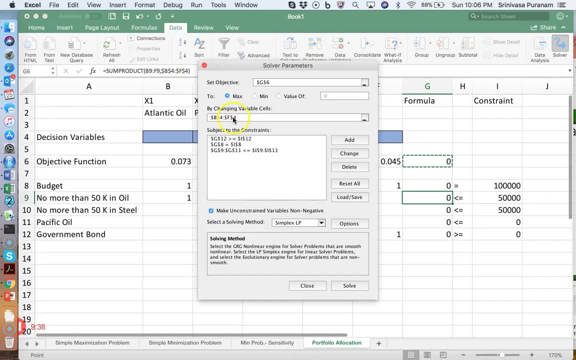 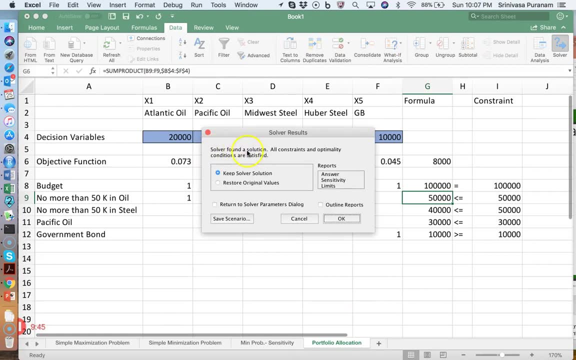 non-negativity constraints are chosen. it is okay. now let me just give you an example. as you can see, I have all of the constraints that should be in place for this solution. the first constraint is the cost of the solution. the second constraint is the profit maximization. I've done simplex LP and I'm going to click on solve. you can. 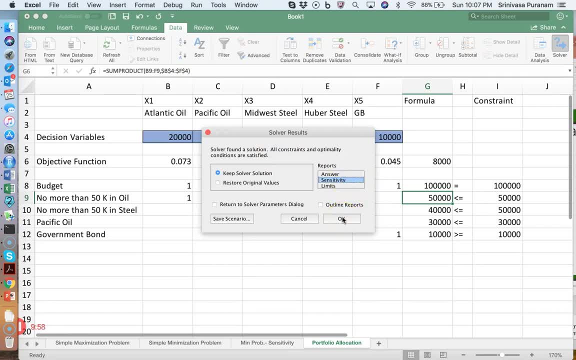 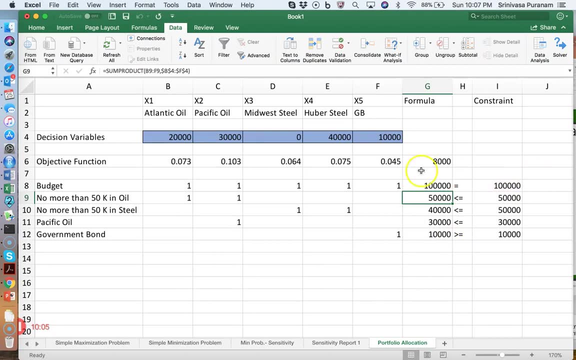 take some time. solve a also call the solution. all constraints and optimality conditions are satisfied and I have all the solutions here. um, okay, I'm going to. that's one of the constraints that you have. so what you're saying is that you're taking the hundred thousand dollars, you're investing twenty thousand in atlantic oil, thirty thousand in pacific. 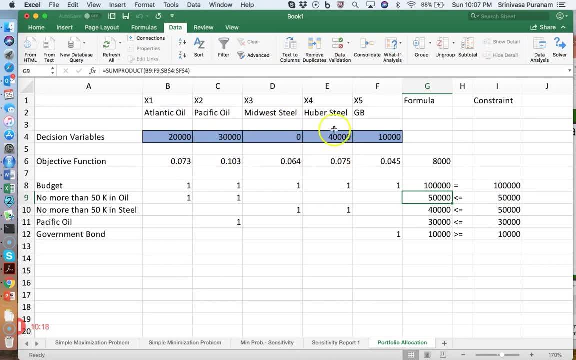 oil, nothing in midwest steel. forty thousand huber steel and ten thousand in government bonds. now, this being zero, absolutely no problem. the final solution just says that don't invest in midwest steel, and that's okay. that's an optimal solution. that is the optimal solution. now the other part. 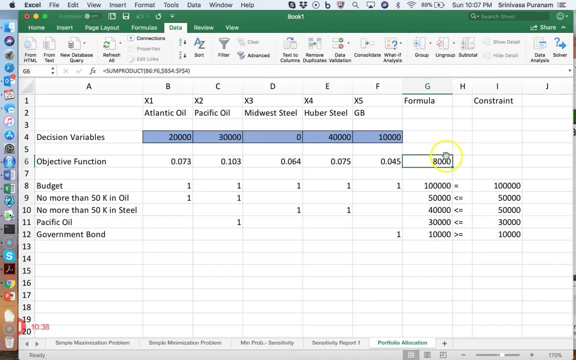 of the optimal solution is that the maximum return that you can expect- assuming that these numbers are are correct- is eight thousand dollars, and you cannot expect more than eight thousand. eight thousand is the absolute maximum interest, that, uh interest- that you can expect from your investments, and that's what you have now. you're using a hundred thousand dollars, so you cannot invest. 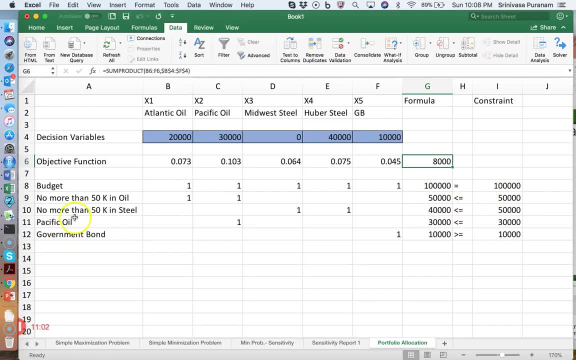 more than 50 000 in oil. you're investing exactly 50 000.. you cannot invest more than 50 000 in steel. you are investing 40 000.. um, you have the pacific oil constraint and the pacific oil constraint and the government bond constraints are satisfied, exactly, specific, all constraints says that you. 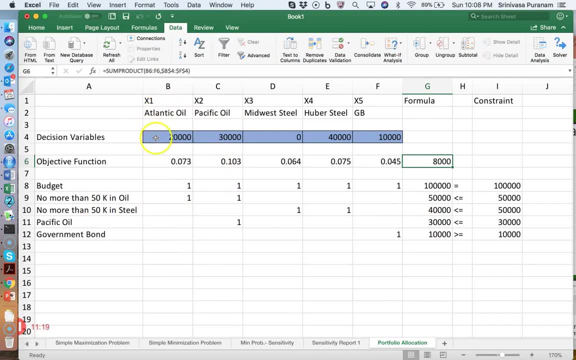 cannot invest more than 60 percent of the total oil investment in pacific oil. so you're investing exactly sixty percent of that. so, totally, you're investing fifty thousand of that. thirty thousand goes into pacific oil, which means that exactly sixty percent of that goes into pacific oil. and